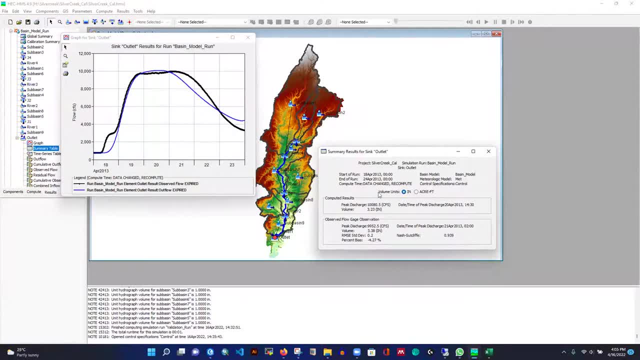 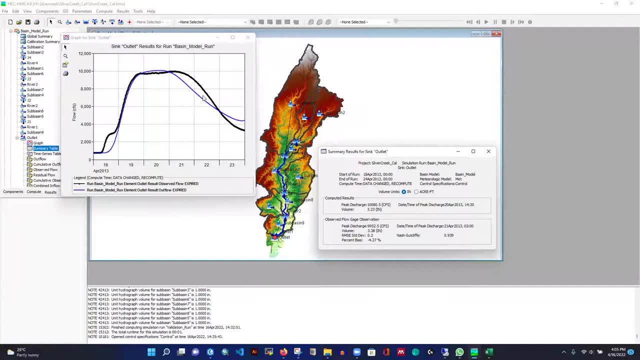 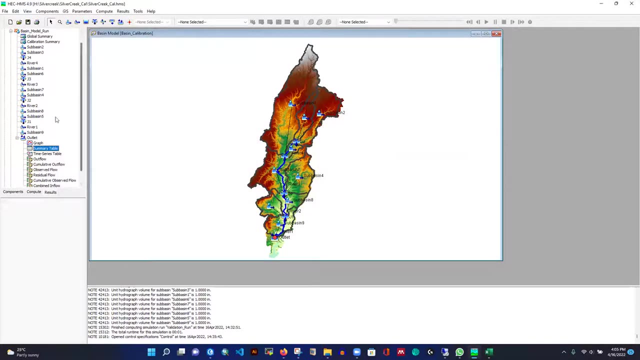 we will change only our forcing. so the main forcing for this model is rainfall, and I have already downloaded this rainfall for another time period- and the streamflow at the outlet as well. so let's see how can we validate our model, since we already fixed our model parameter in our calibration right. so I have just 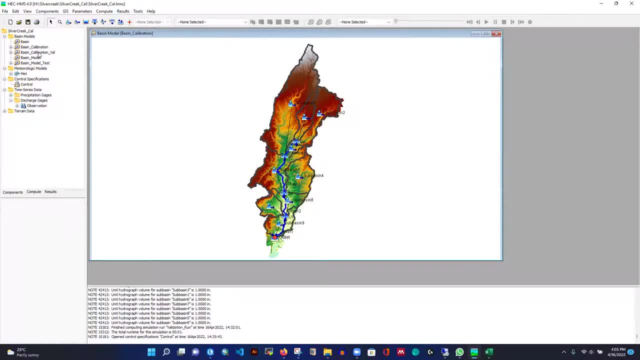 copied this calibration, basin calibration, as basin calibration underscore valve. so this is for validation and, yeah, you can just right click and you can make a copy and you can just rename it. that's it. so this is how I just made this copy of our basin calibration and then what I have to do: I 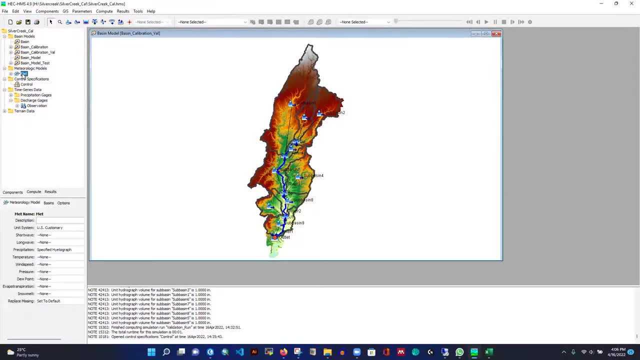 have to add my met model here. I have only met model for calibration. I'm gonna add another met model for validation and then I need to generate controller specification and I have to add like time series specification and time series charge. so let's see, from component I can even create metallurgical model. 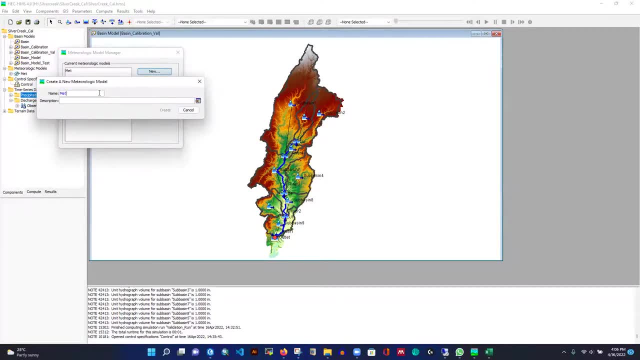 manager, and then I can click new, and here I can rename it as Matt and Val- okay, and then I can give the name as like: validation- okay, validation, and that's it. okay, I can just click OK, that's okay. and then what you have to do if I click there? 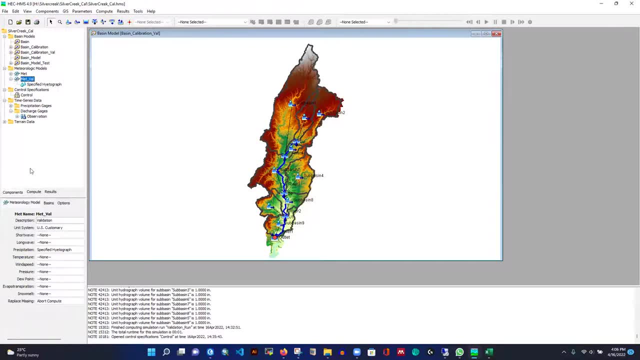 see I have this right. so here from basin, and I can even change that on me if I have any missing values or don't abort. instead of doing that, set to default and then see: from basin, I have this right. basin calibration. well, means that that is my current basin, so now it is no changing it to yes, so that means my met. 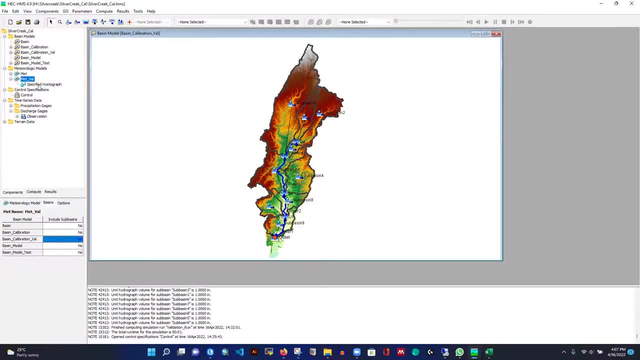 model is connected to my basin model and then if you click on the specified height of graph, see, you can see that it is not connected. so we have to generate rainfall time series. then we will get access and then we'll add that, because the one we have it is for calibration period. so here from 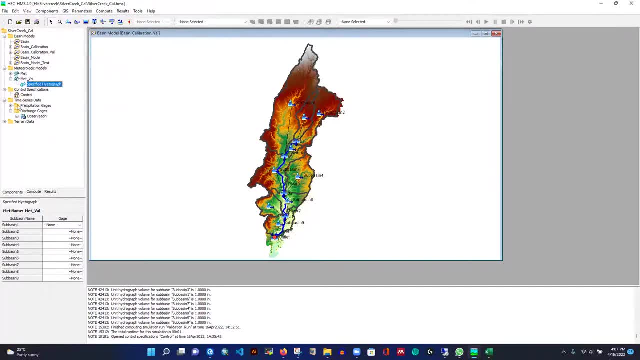 component click on. okay, instead of doing the same thing, I can just copy. okay, I can make a copy of that. I can right click on that and then create a copy. then I can change the time. so rainfall, so I can as well. so this is for validation: rainfall, okay. 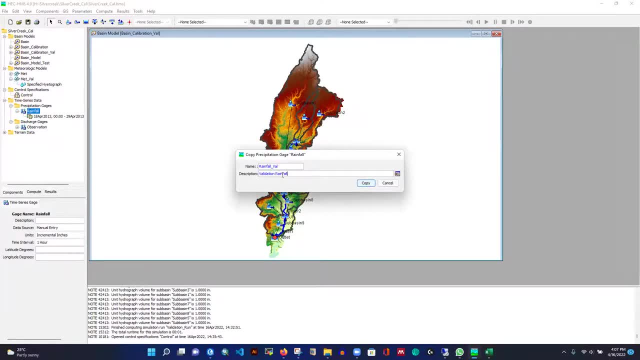 validation: rainfall series. that's it. so I have the same time. but let's check. and for even discharge, I can even copy that one as well, because I have the discharge data as well. so observation for a validation file: okay. so observe, discharge for validation: okay, so I'm creating the copy. I have that data set. let's populate this time. 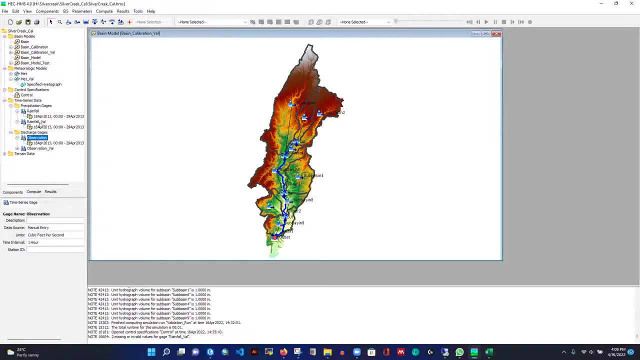 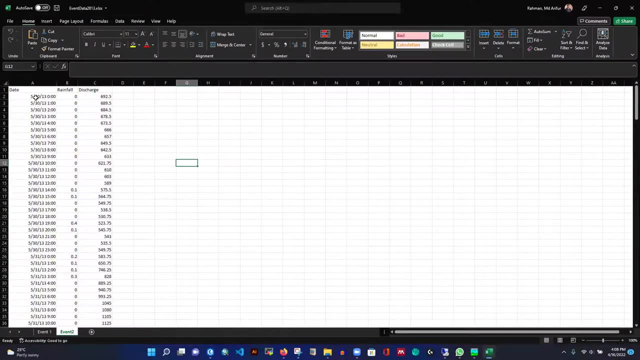 series with or for rain fall. the time will be. I have the excel file here, we can see it. the time is inches of rainfall, the timelen, the time is, then the flow rate is basically cfs mixed with the speed苗 vhey literally mean the time series, time series foo latest, which is really capitalized. okay, moment to play and say, or first timers, once an hour you have first little and reason to time result on the key requesting time series: okay, and again, we booked that time series. I had проис. so what we did at the extent itself. this a simple little review of that decrease. okay, stink in special case. this will actually 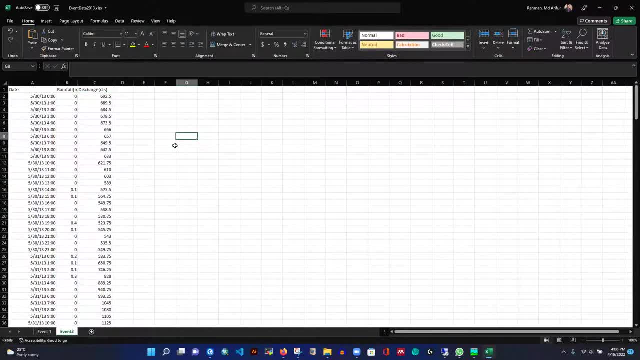 CFS, because we are using CFS. if you already saw that previous video, then you have idea about that. so the time from May 30: 00 hour to all the way to June 9, right and 2013 and the hour is 5. okay, so let me specify the time there. 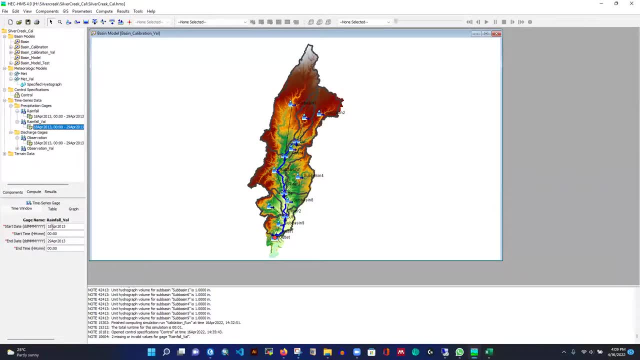 that time. here. here we have to change it like 30 May right 30, 30th of May 2013. it is same and we calibrated the model for the same year but for different time period. for April, you can see the time, and to 9 right June 9, 2013. but here it. 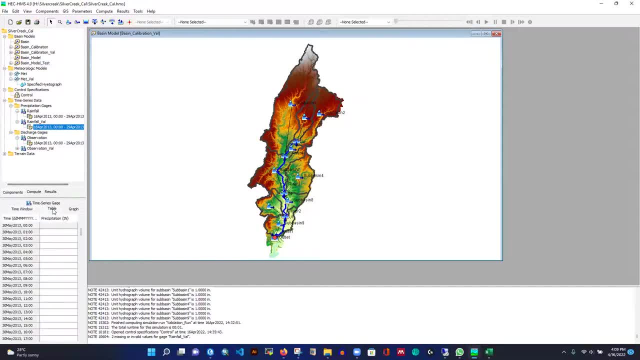 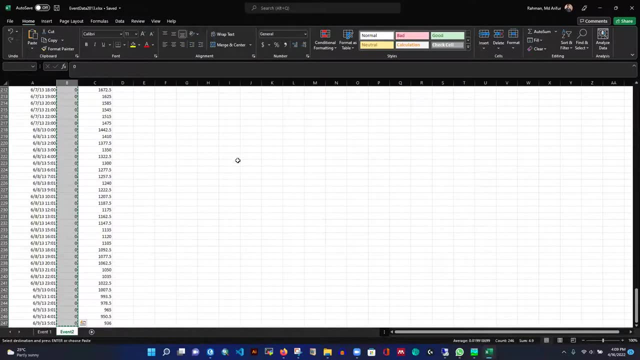 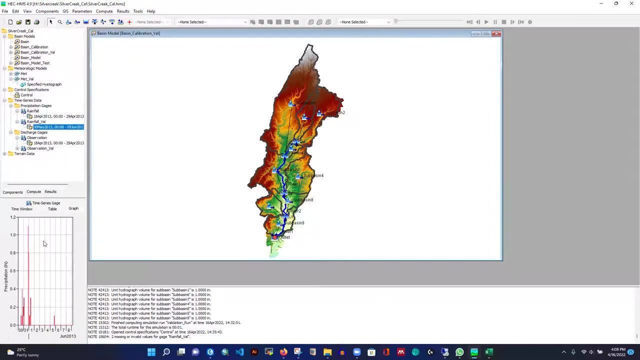 will be 5 hour then I'll have the time, since now what I have to do, I have to copy time, see the series. then I can even paste it there and I can even plot it. so this is my rainfall data set I just imported and now do the same thing for discharge. so for discharge, okay, let me check that. 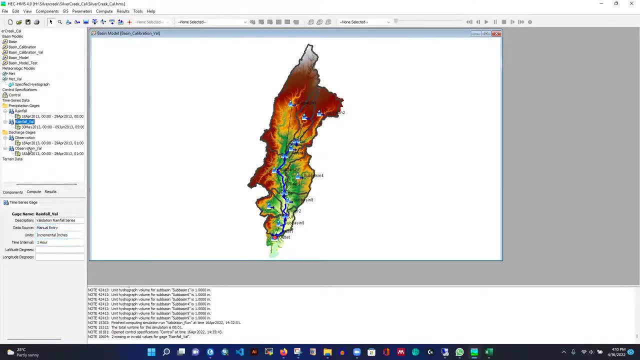 even again. so it is incremental inches, all the data, everything looks okay. that's why I copied, so you don't need to fix it again. so it is same. what I have to do is I have to copy the time series and then I can even paste it. 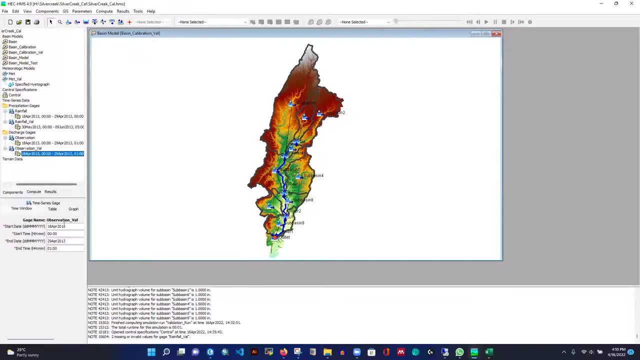 one hour and cubic feet per second, and then I can change the time. it is the same time: 30th of May 2013. 00 hour to June 9. okay, June 9th June 2013, but instead of one hour, it is going to be fifth hour. then we have empty table and 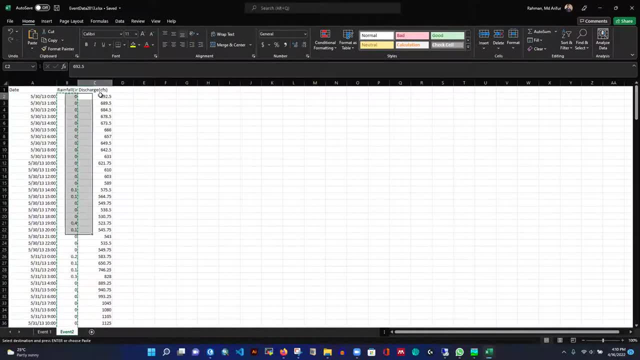 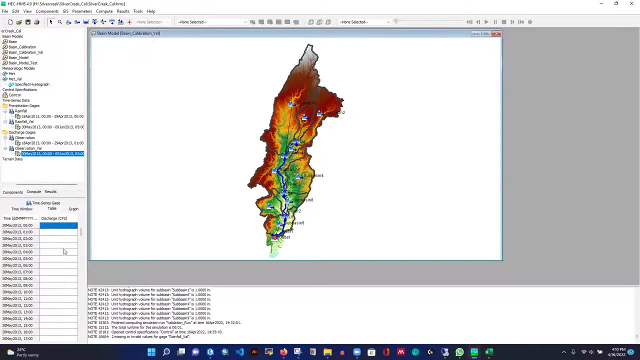 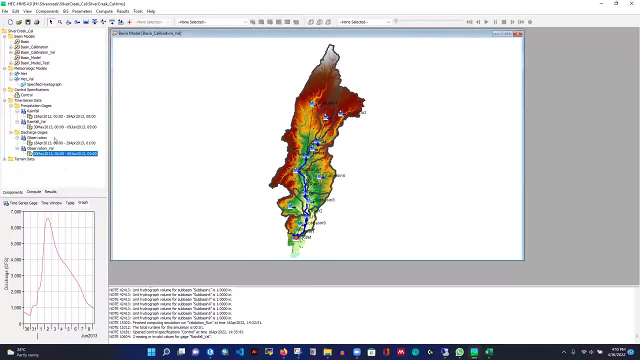 here we can even copy the flow rate. so what I have to do is I have to copy the time series and then I can paste it there. so that's it. you can see the graph, okay? so this is our graph now. this is it. so we have our rainfall, we have our flow rate, and what do you have to do? we have 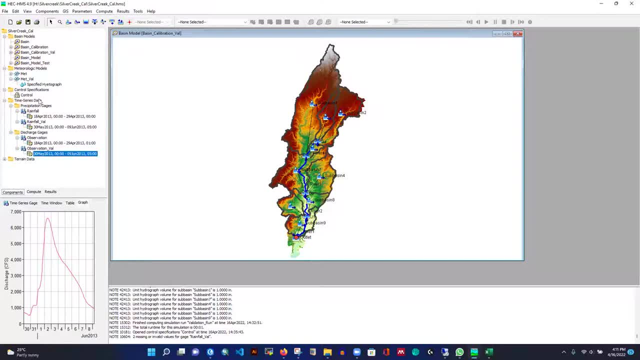 to connect this observation well, to the outlet, right? so let's go to that: basin calibration, not calibration. this is basically okay. let me rename that I'll. i just copied it and i added file, but it should be different, okay, so validation: okay, basin validation instead of calibration, valve validation. okay, so that's it, and now maybe i have to change. 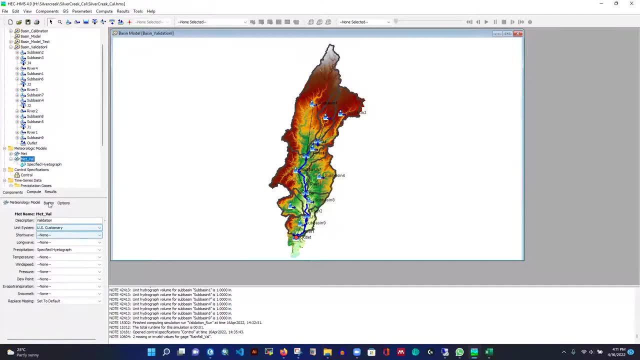 that matte model, because it is going to be different. this matte model, uh, yeah, so we have validation. okay, i made some error. okay, okay, now it's perfect. then go to this one and check that. if it okay, it's yes, no problem. then what you have to do here, you can find that time series right. 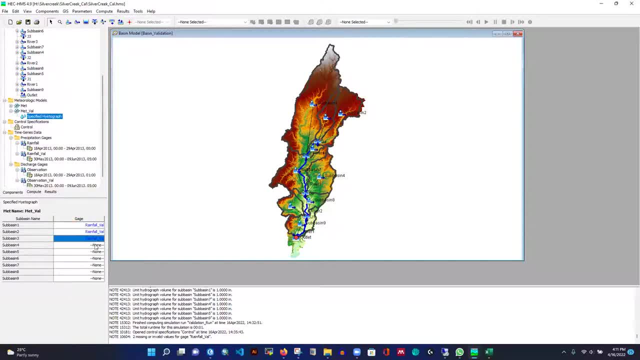 rainfall val. select that this because this rainfall. well, we have only one station observed data. that's why we are just assuming, okay, we have rainfall everywhere from this data. so this is a little bit problematic, but we don't have any option to do that and we did the same. 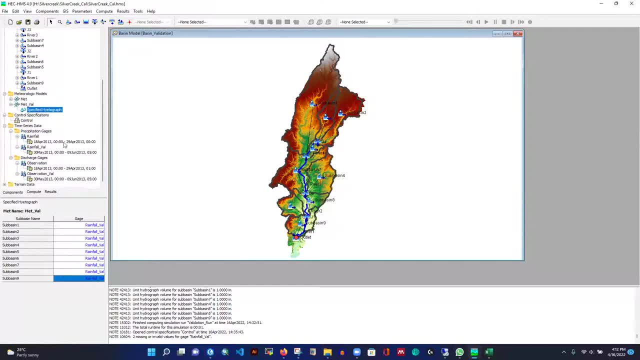 thing for our calibration, so we are going with this one. whatever data we have, and we have this observation, let's connect the outlet with the observation we have. uh, from validation. so here option, select that observation. well, so our outlet is connected to our observation and then we have our rainfall right for this 30th of may 2013 to 9th of june 2013, and 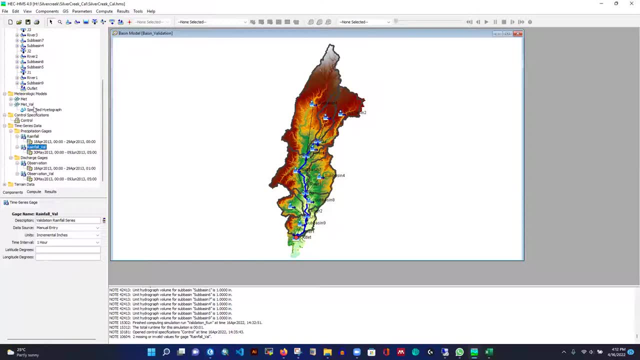 up to our five. so we are done with our met model, we are done with our time series. and then what we have to do? we have to create control right, controller specification, and then we have to create the run simulation. so for the controller specification, this is for calibration period. then we can even copy that and change the date and time. 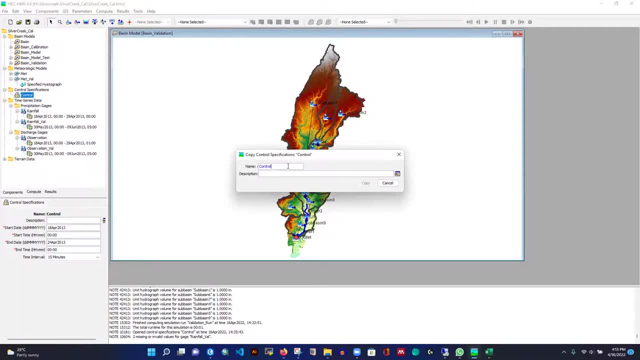 so create a copy. and this control is for control underscore. well, okay, so we can describe that. okay. control specification. specification for validation period: right, yeah, and then this control is has the same time, but we have to change it like 30th of may, 30th of may 2013, 00 hour to june 9.. 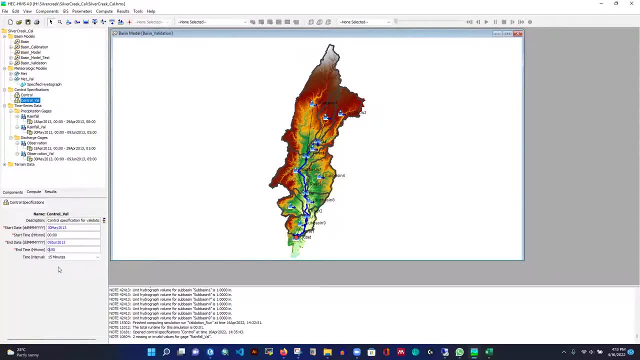 so 2013 and up to this fifth hour- and this has to be like one hour data. because we have hourly data set, we can even run for lower time period as well, but since our every data observation data set is in hourly time and steps, so we can even go with the same time and stuff as well. right, 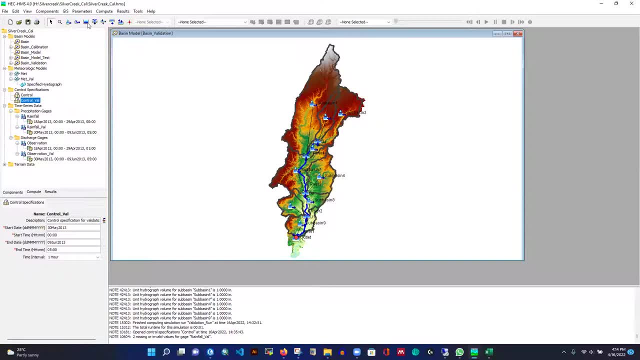 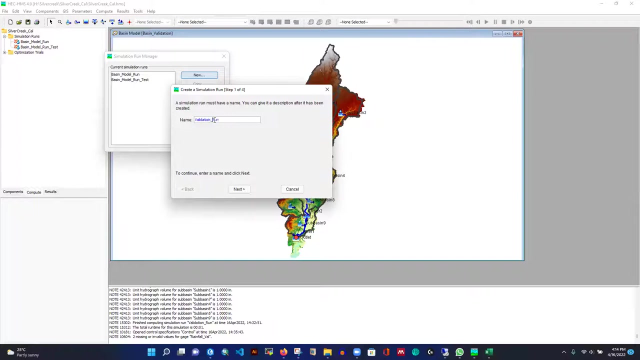 so we are done with our control specification and what we have to do compute. so in our compute we have to create the simulation run. so go to compute and simulation run manager and then create a new one run called validation run. okay, validation, validation run. and here we have to select: 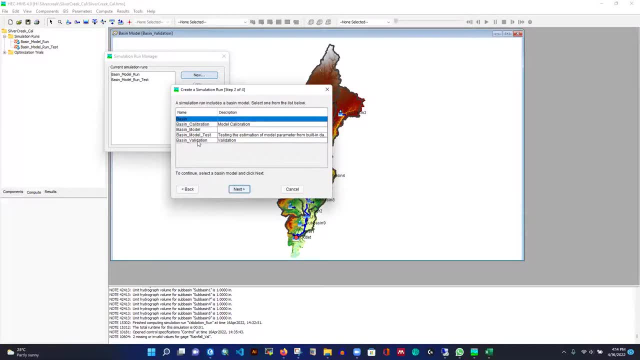 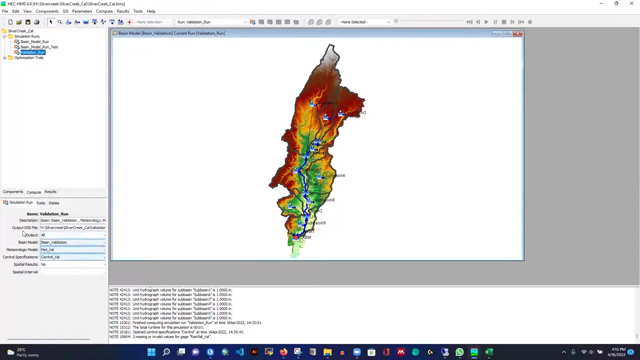 that basin model for which we are going to validate our model, so base in validation- and then the met model. we have to select that met model for validation period. then we have to select the control specification for validation period. so we are done with our uh simulation. right here we have that. so we can see that okay, output will be all model is. 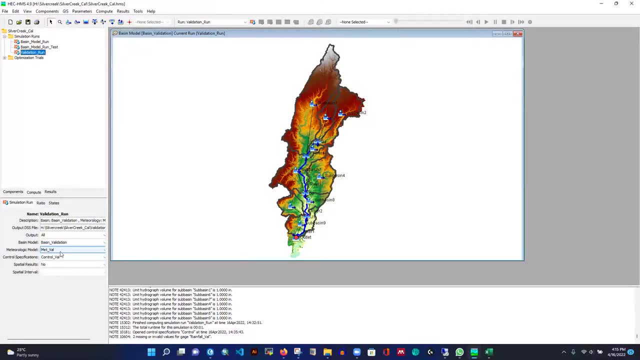 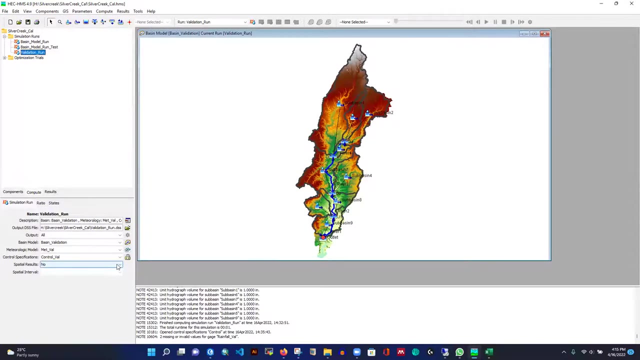 based in validation. our metallurgical model is met validation controller specification is this: and if you want to even write the spatial result, you can see that that is also possible and let's see, yeah, if you want to even show like special result, like especially distributed rainfall or anything else. so we usually do this for the gridded model in a. 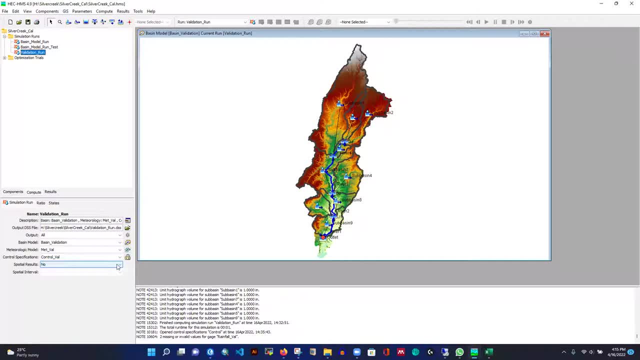 my future video, i'll show you how to set up a gridded model instead of lumped model, and then i'll even turn this on and then i'll show you how to show the results as well. it will show the especially varying rainfall run of everything, okay. so now we're done with everything. i'm just 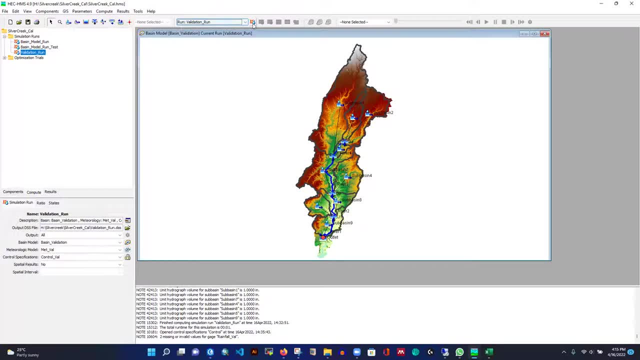 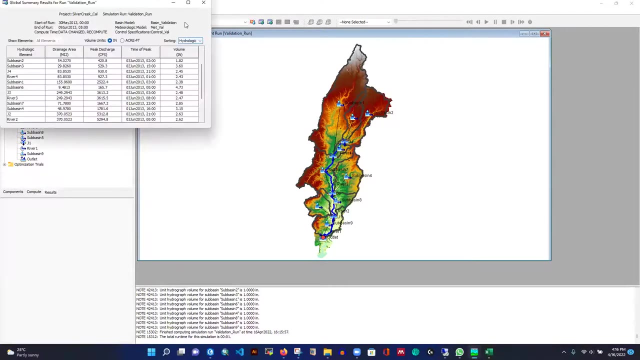 setting the model and now i'll run it- validation run- and then we'll see our result as well. i don't know what is going to happen. it runs pretty quickly, go to results and this is like different run. we have so validation run, click there. it's a global summary. you can see that this is our 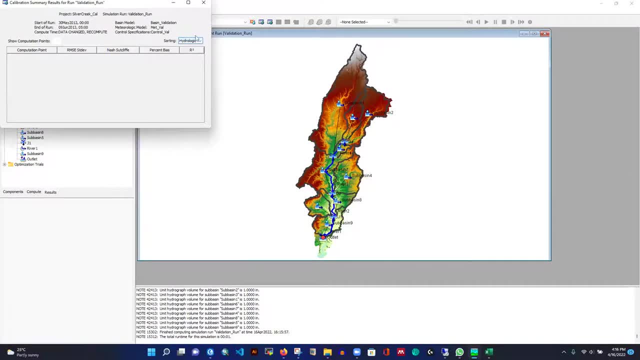 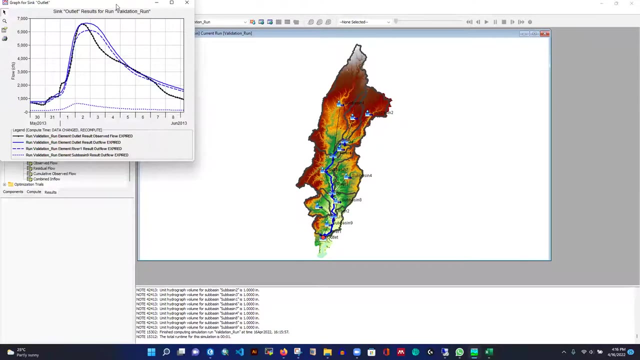 global summary. and then we have this summary. there is: there is nothing, because we don't have any observation for each of this. we have only one observation there at the outlet. we can click there. we can see the graph. oh, it's really looking good. okay, let me just uh remove the other one and let's see. 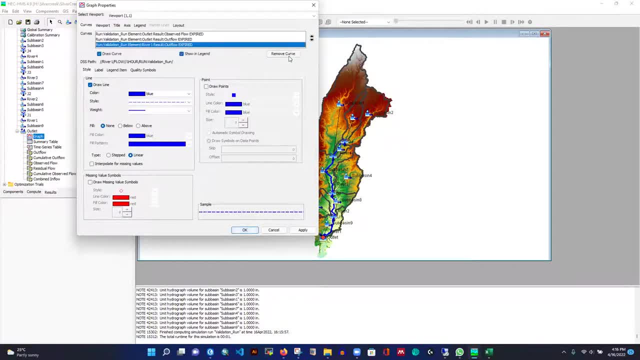 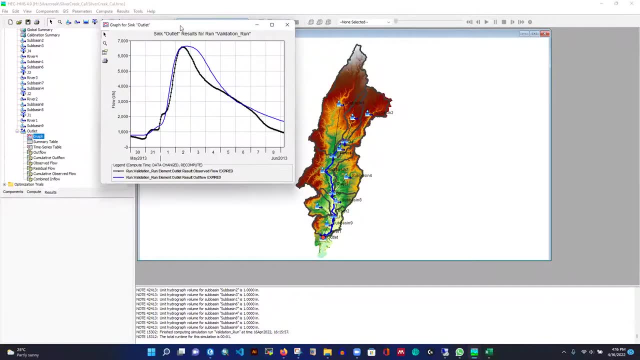 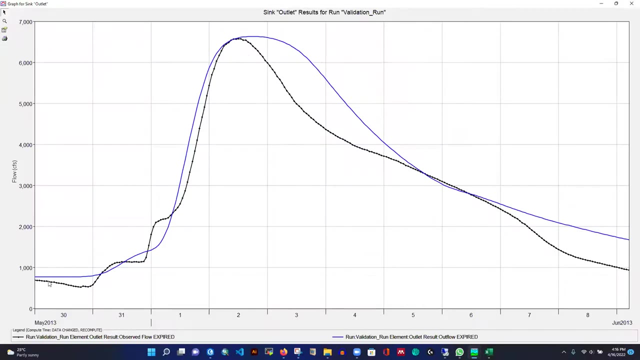 actually which one we are comparing with our observation. i'm deleting extra. yeah, so that could be our comparison. okay, so this is our validation. it looks really good because our calibration was good. right, it is clearly capturing the peak and everything looks okay. okay, so that is the validation. 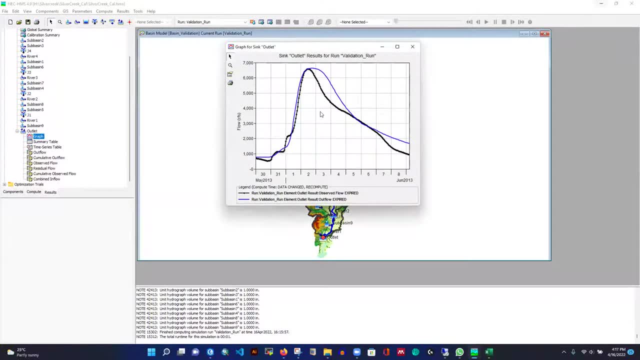 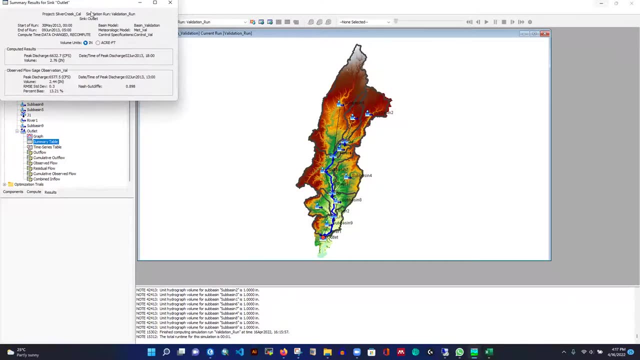 okay, so that is the validation among. okay, so that is the validation among. it is: it is expected that the validation result should be reduced compared to calibration, but i don't know what happened. let's see, uh, table summary. right, oh yeah, so it's like 0.893 the. 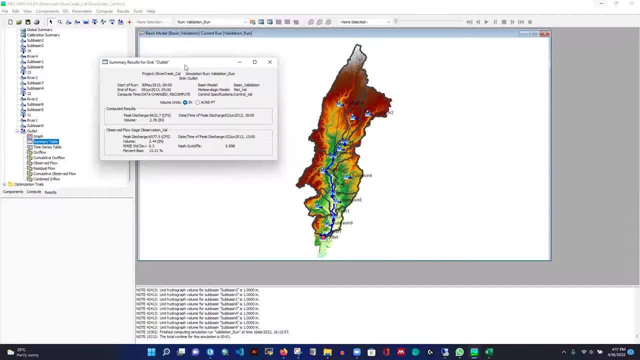 nesh shirtcliff coefficient is this and the percent bias is 13.21 and the volume is 2.44, but our volume was 2.76 and that's okay. and in terms of like peak discharge, we have six percent of the peak discharge and we have six percent of the peak discharge and we have 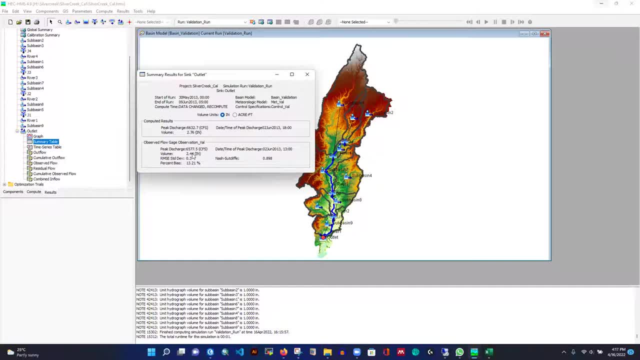 66, this is the computed 6600, and here we have 65, almost 666, right, it is 6577, and that is like 6632, almost the same. and here, in terms of the timing, uh, june 2 2013, 18 hour. and here it is like uh, 13. 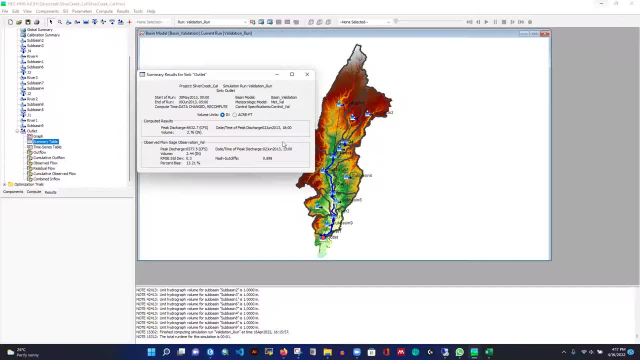 hour. so we have like five hour difference. that's okay, it doesn't matter, but still it is capturing pretty accurately. and the go, that's okay, it's okay. it's okay, it doesn't matter, but still it is capturing pretty accurately. and the correlation is too good. and if i compare with validation, let's see if i have the results. so 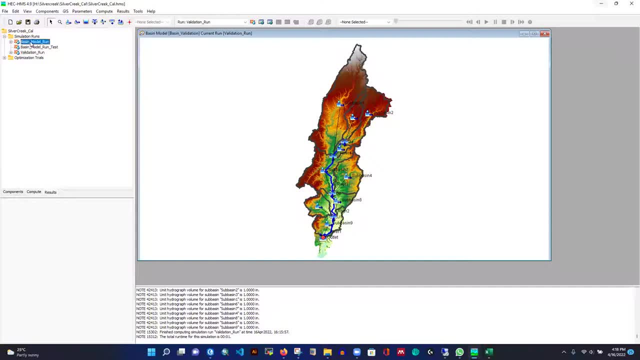 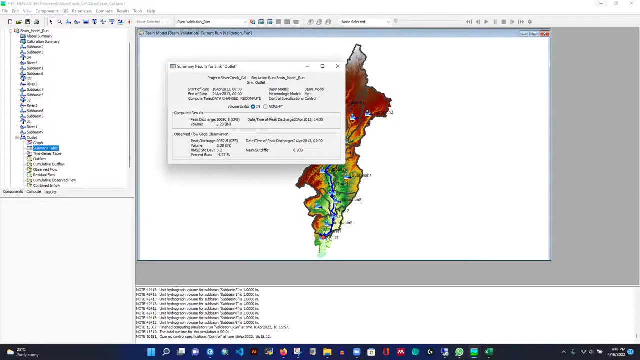 maybe i'm reducing that. that is my validation, right? yeah, so that will be okay. 939, let's compare with calibration and the validation. so that is calibration and that one is a validation. so it is particularly good and dedicated to the. there we go, okay. so at the end it is 0.939 and it is 0.893. it's almost same. if you compare the percent bias, it is around 5 percent minus 4, it is 13, and here the rmac is 0.2, 0.3. 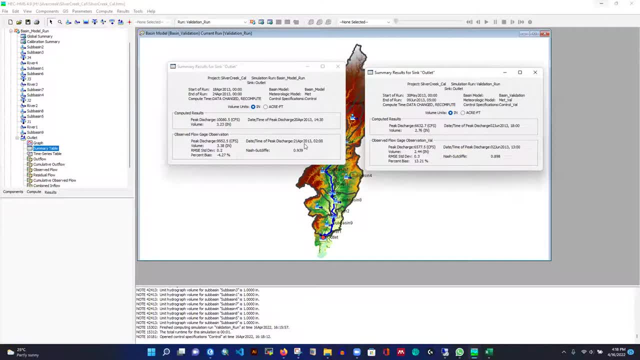 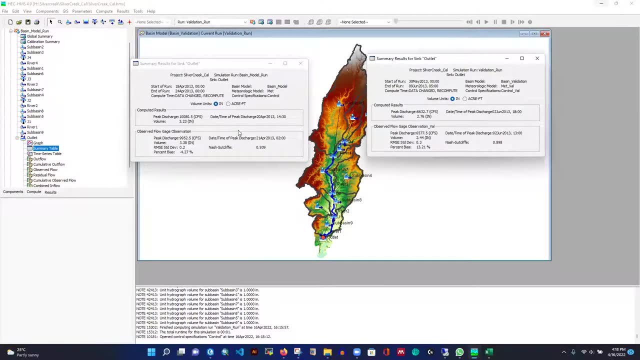 that's okay. so in terms of correlation, this calibration and validation looks pretty amazing. so if you have a model like this, your calibration is too good- like this, more than than 90. and if your validation also same, like more than 90 or close to 90, right 0.9, that means your. 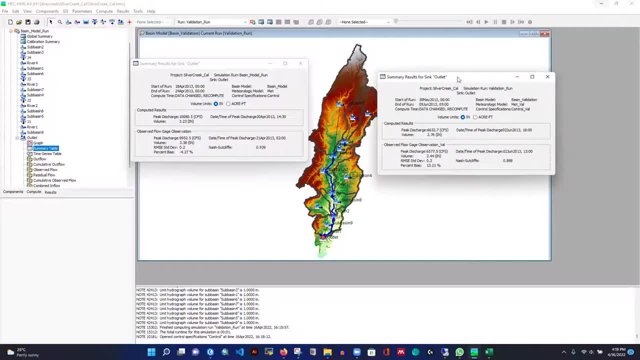 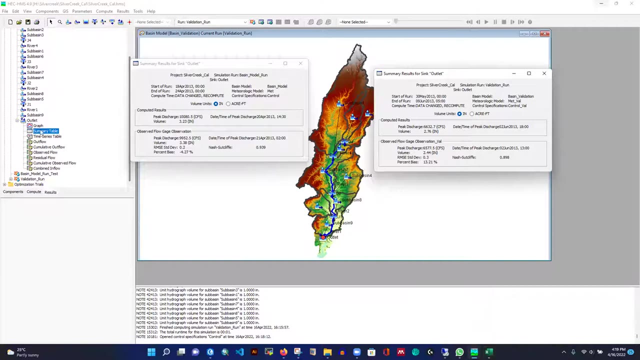 model is very, very good and you can even apply this model for any other event with high confidence level. so this is how you can even validate your model. and if you want to even check other criteria, other properties, then you can do that. and if i compare the graphs again, let me even remove. 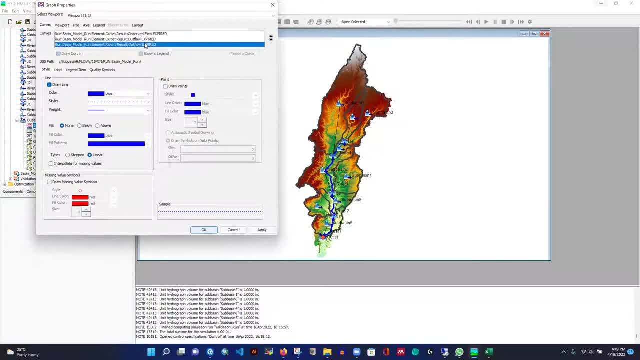 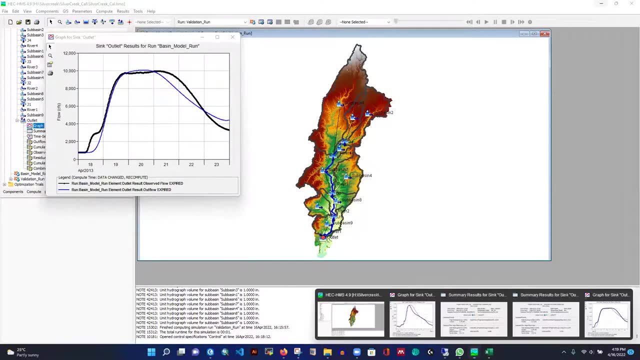 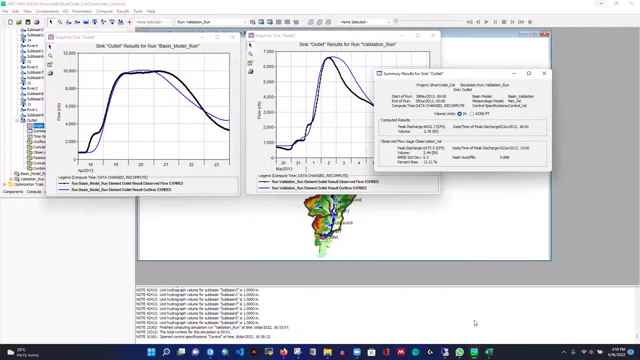 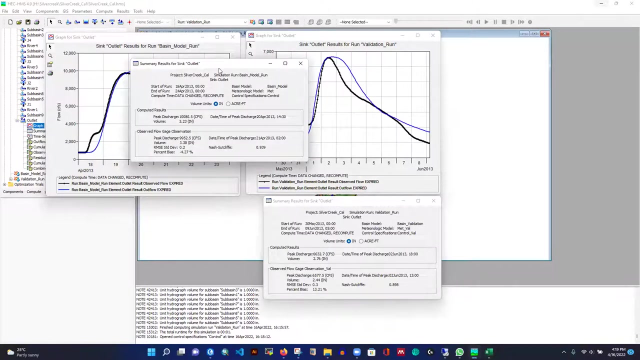 and clean it, removing the local flows, and we have this graph from calibration, we have this graph from validation, right, and we have? okay, let me open that table. this table is from validation, and we have another one. this table is from calibration. so that's it. so this is the 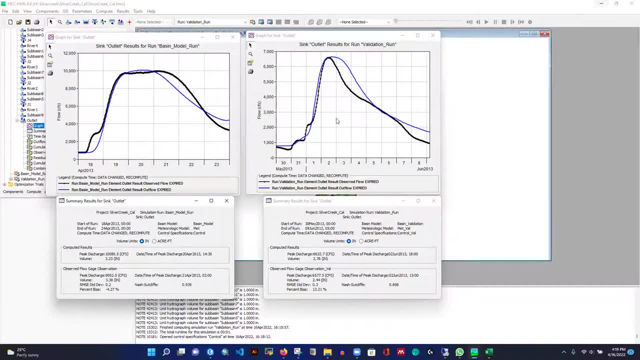 calibration curve and the statistics we see. and this is the calibration curve and the statistics we see. and this is the calibration and the statistics we can see. so it's pretty amazing because this model is kind of challenging. see, the calibration graph is kind of flat. the hydrograph observation hydrograph is. 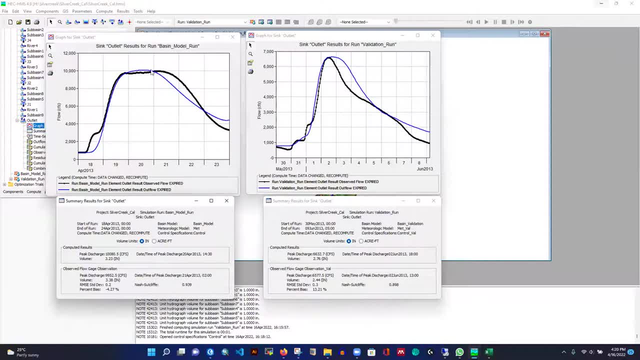 not that typical hydrograph. rather than having a sharp peak, it has a flat peak right. that is challenging to capture and still we have, like, good correlation and for validation period. if you have a good correlation, you can see that the calibration curve is kind of flat. if you have a good correlation, you can see that the calibration curve is kind of flat and it's typical. 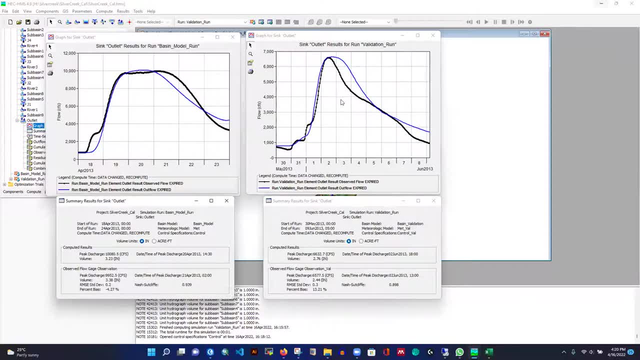 and it's typical hydrograph we usually see in any flood event. so so what are the process to your hydrograph we usually see in any flood event. so so what are the process to your process is to validate any model. so if your model is calibrated, then just copy the basin model, because we have to keep right all the 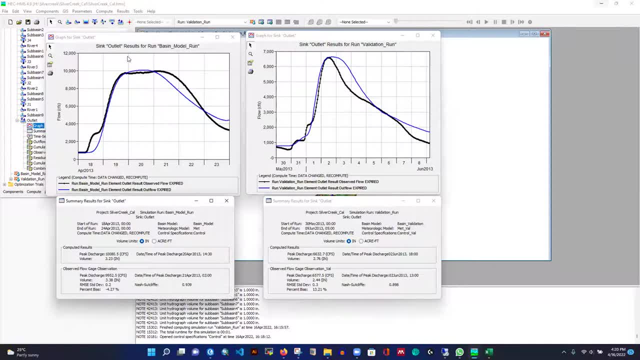 calibrated parameter. so that's why you don't need to change anything without changing any model parameter. just copy the basin model, then use different data set for different time period, the time series data, like all these four things, rainfall, and if you want to even check, you have. 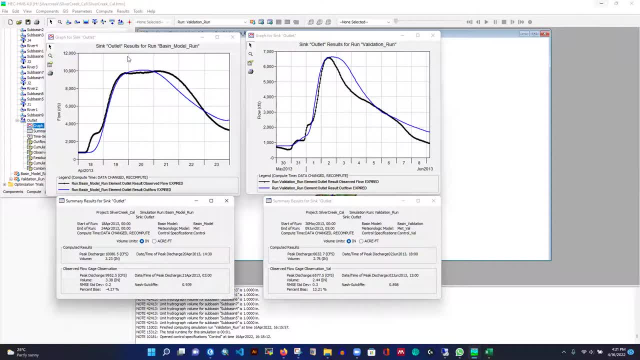 to have, like observation data set right for the same time period, means for the validation time period. and then, if you run the model and then check it, if it like uh, within your expected values, like more than 0.6 up to one, the more the better- then you have your model ready. so now you have the tool ready to even run for any other event. 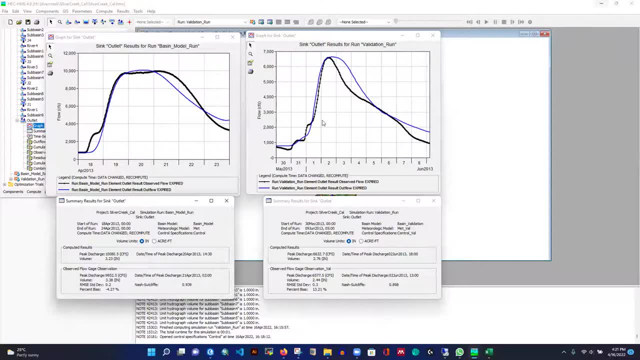 so now our calibration looks good, validation looks good, so we have the tool ready on our hand and if i see that, okay, i have one event and i can even run it. okay, so that's it. even if you wanna predict, uh, some future scenario when we can do that, there is also possible that you have any candidate. 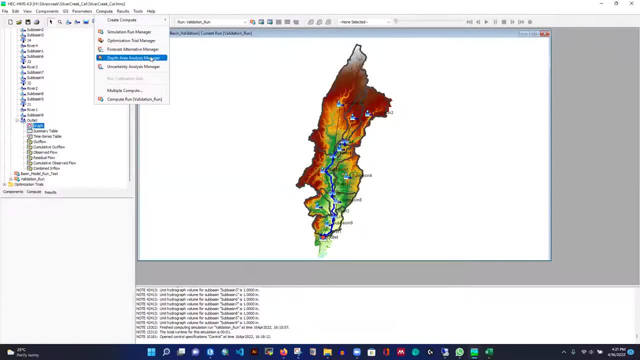 possible. maybe in my future video i'll do that, so from here we can even do the same thing: forecast alternative manager. if you even click on that, that is also possible. then what do you have to do? you have to create the forecast one and for like validation. okay, since i have validated the model. 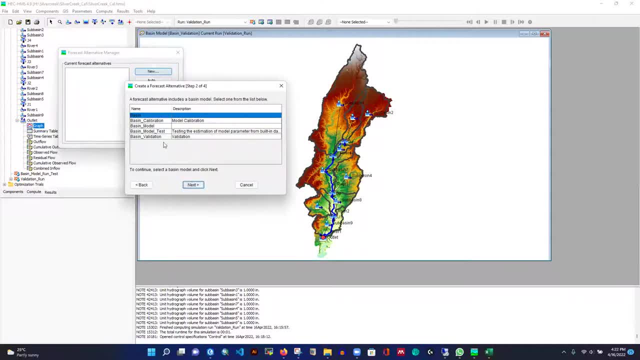 i can do that, and for calibration, even i can do that as well. okay, for example, for validation, i can check it, and then for met model, you can select anything. that is also possible. so i'll show you that in my future video- how to even predict future condition using this model, because our tool is now 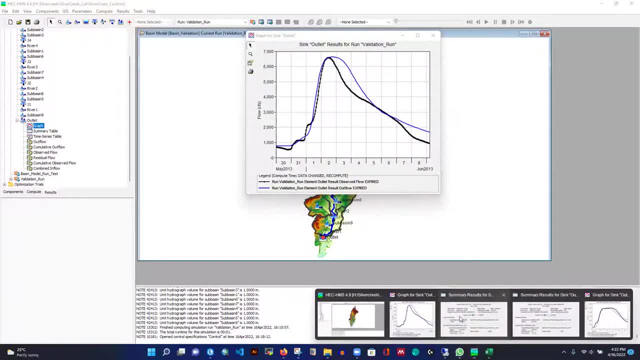 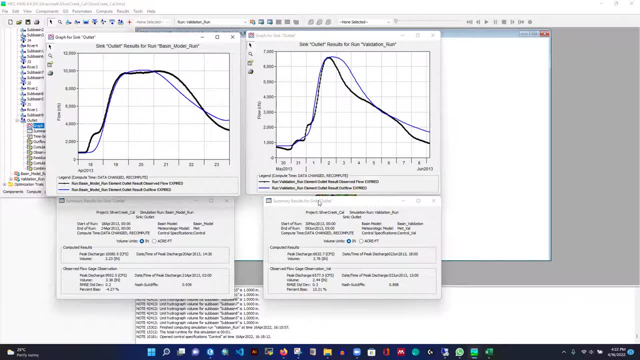 ready. so that's it. we have everything ready like this, and you can even practice for your study area, and let me know if you have any query or question. i'll try to answer that. so until then, stay safe and thank you very much for supporting my youtube channel.